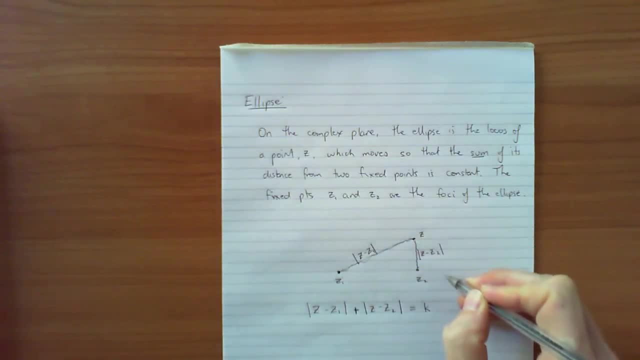 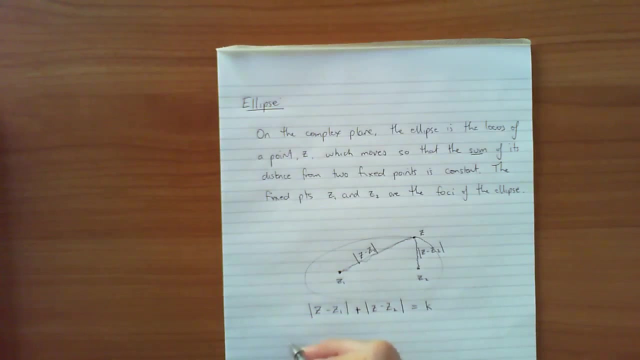 And then we moved our pen around, keeping that string tight. What we would actually do is we would form an ellipse With z1 and z2 being the foci. Now a couple of useful things here to note. k is actually the length of the major axis. 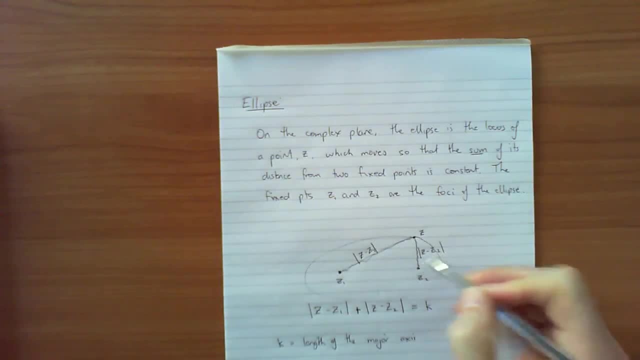 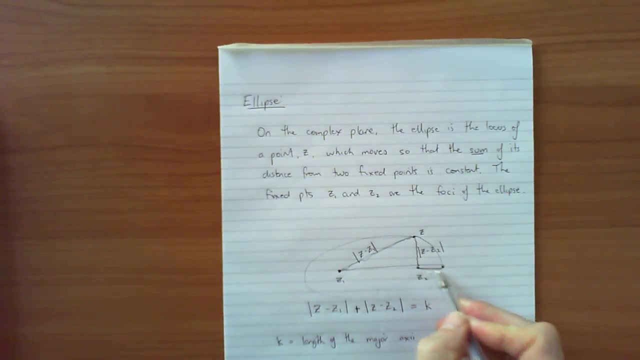 k is this length plus this length. If you imagine when you, When your pen is out at this point here, right at the vertex of the ellipse, the string is going out here around your pen and back to there. If you were to imagine this, you could cut that little bit off there and place it over here, and then the string would go from one end of the ellipse all the way to the other end of the ellipse. 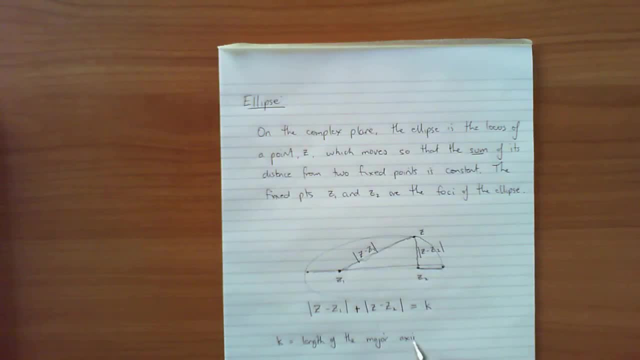 And then the string would go from one end of the ellipse all the way to the other end of the ellipse, Which would be the major axis. So k is like the length of your string, That distance plus that distance, And it also then is equivalent to the length of the major axis. 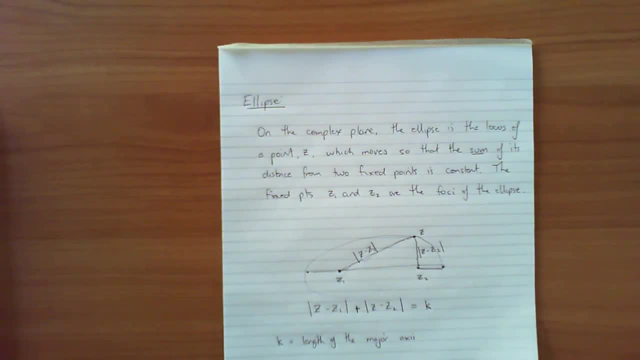 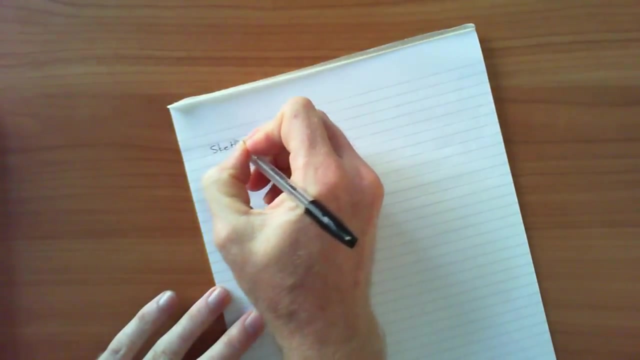 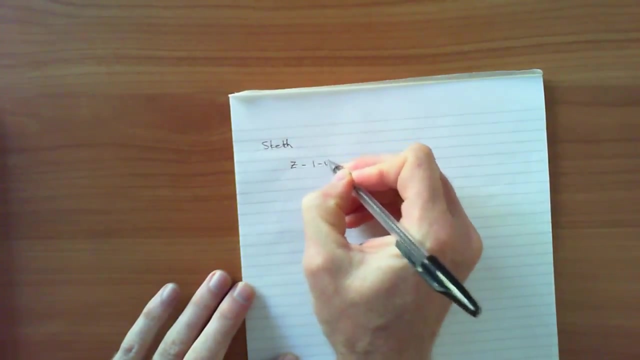 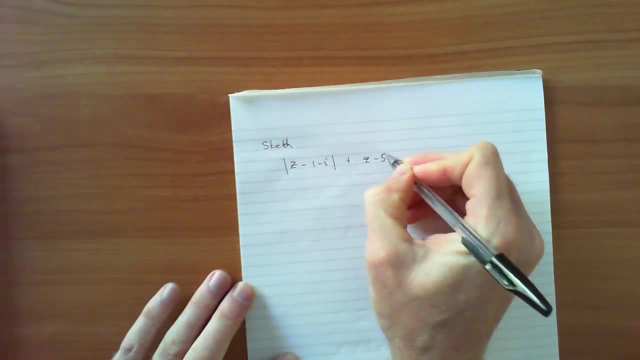 Okay. So how do we actually sketch an ellipse and show the key features? Well, let's look at an example of that. So we're going to sketch z minus 1 minus i magnitude, plus z minus 5 minus i magnitude equals to 6.. 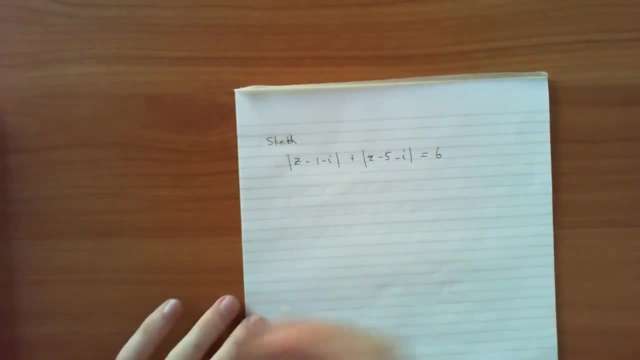 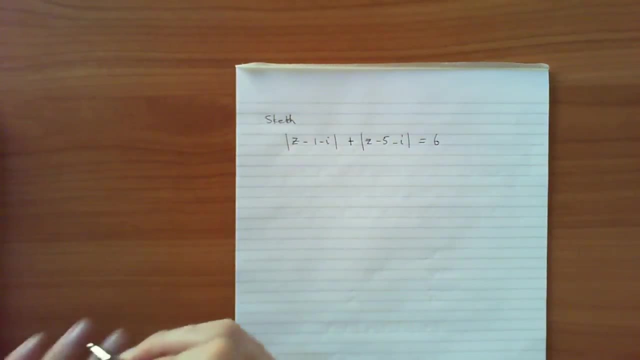 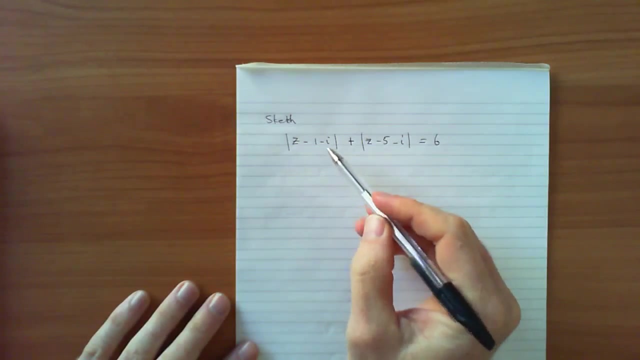 Okay, First of all, we need to, First of all, we need to recognize that this is actually an ellipse. We know it's not a straight line because we don't have one distance equals another distance. We know it's not a circle because we don't have magnitude equals a constant. 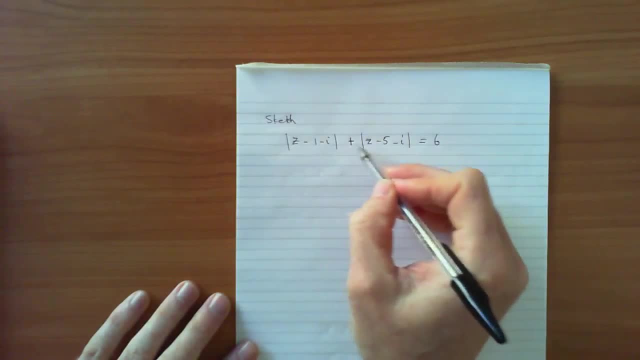 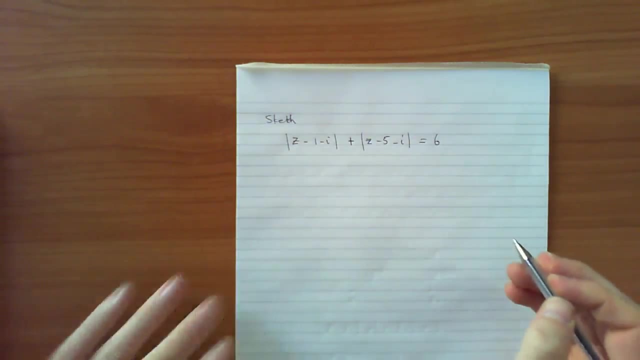 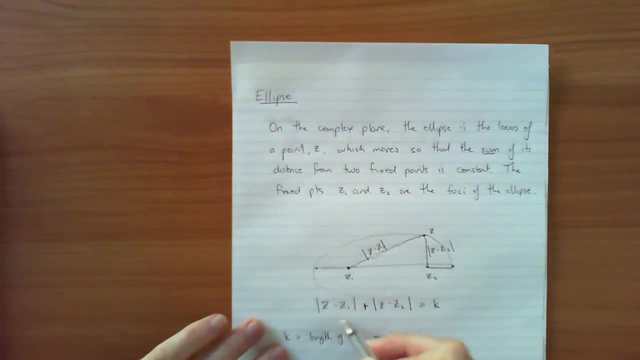 We do know it's an ellipse, because we've got one distance plus another distance equals a constant. So that is the standard form of an ellipse. But remember that the standard form is, as always, z minus z1.. Because the distance between two points is subtracting them. 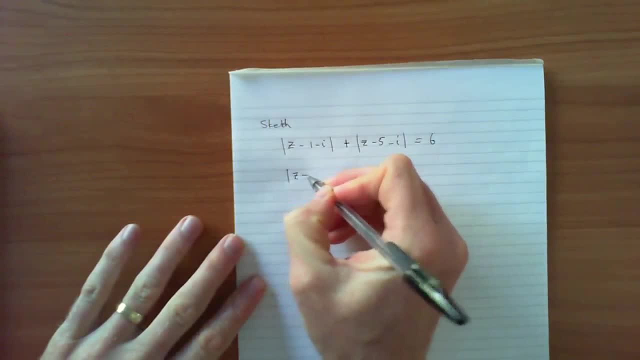 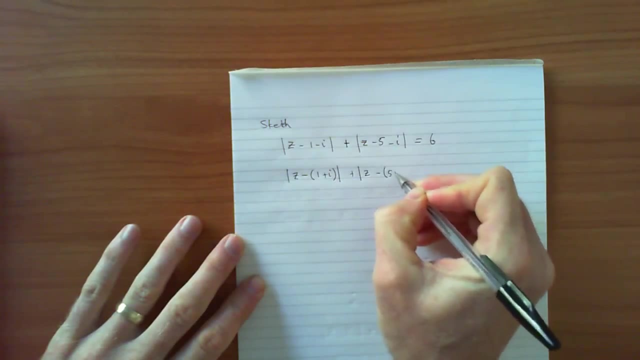 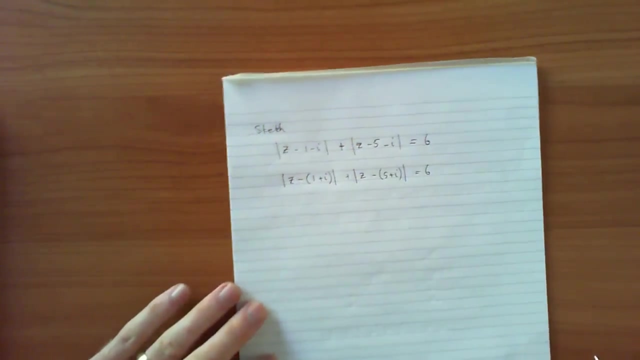 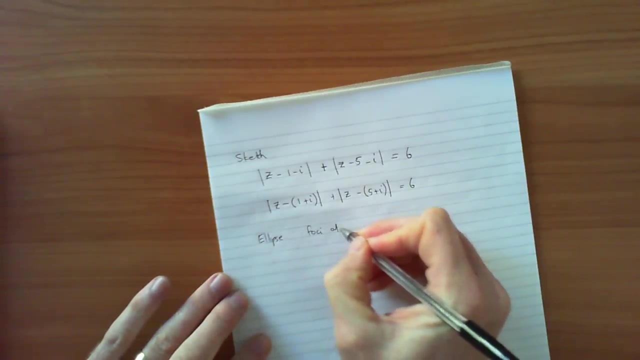 So to put it in standard form, here we'll have z minus 1 plus i plus z minus 5 plus i equals to 6.. So we know this is an ellipse. So now we have foki Foki at z1 equals 1 plus i. 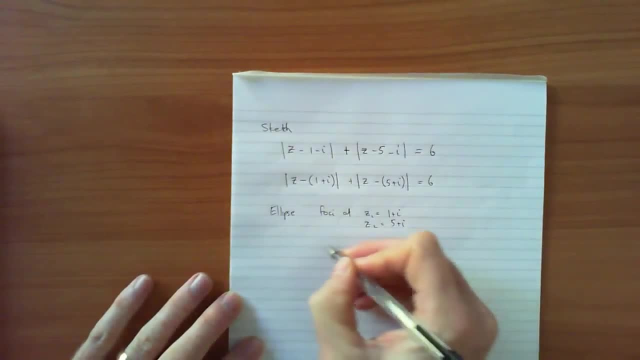 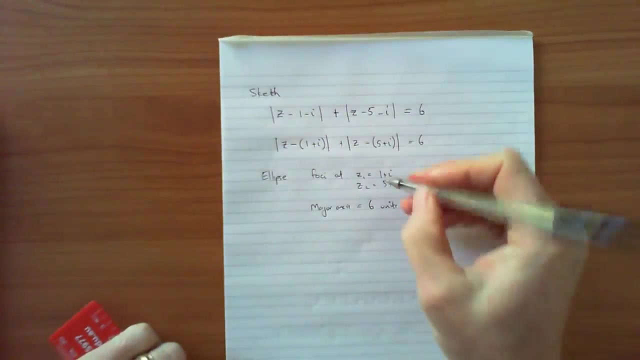 Z2 at 5 plus i. There's our two foci And we know our major axis equals 6 units. So when we come to sketch this, this time I probably will use a ruler. We've got foci at 1 plus i and 5 plus i. 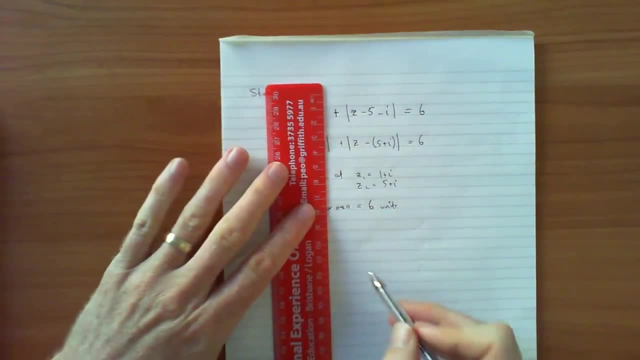 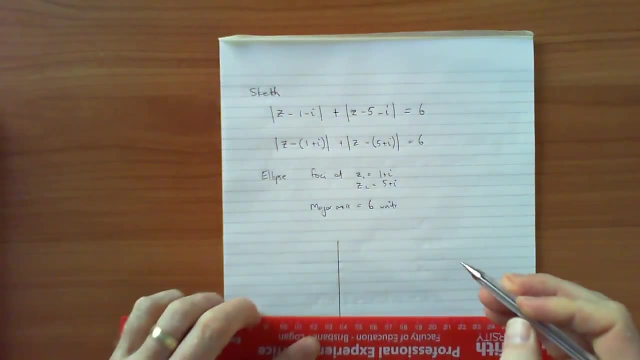 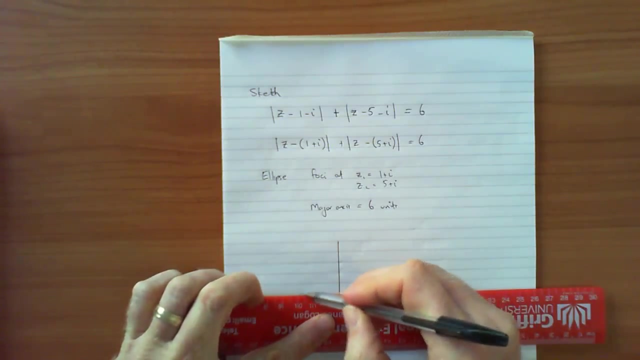 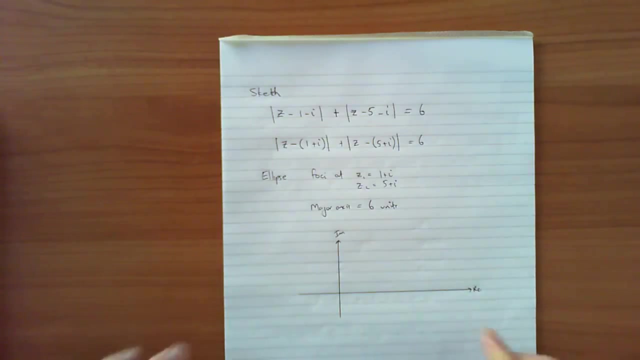 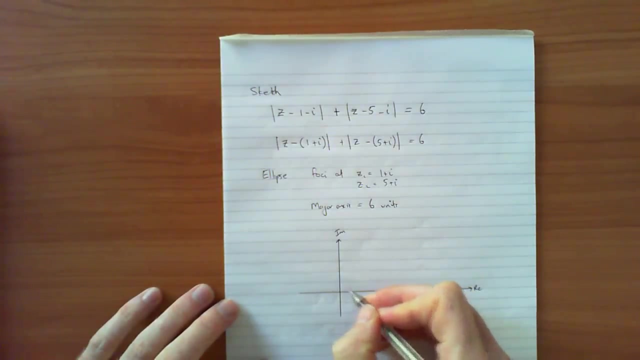 So if we do this, and 5 plus i, So we're going to need a little bit more on the right hand side of our graph, Imaginary, real. Okay, so we mark on our two foci. that's the first thing we can do. So at 1 plus i, which will be there, and at 5. One, two. 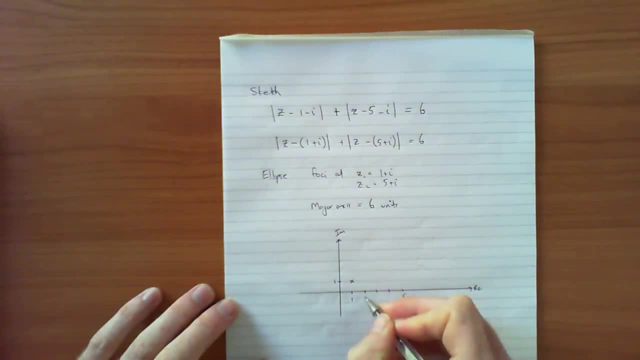 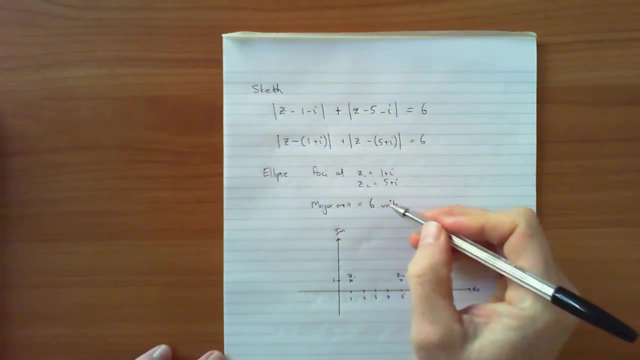 three there. those are our two foci: Z 1 and Z 2.. Now, if we've got a major axis of six units, in order to mark the major axis on, we first of all need to know where the centre of our ellipse is. 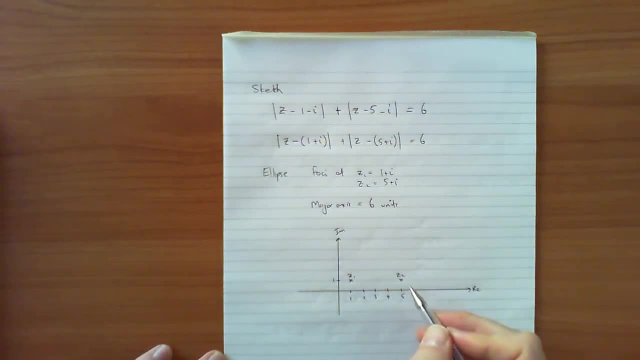 now, in this case, if your foci are here and here, we always know our centre is halfway between the two foci, so it's pretty easy to tell that the centre is going to be right there, if it wasn't so easy to pick for some reason. 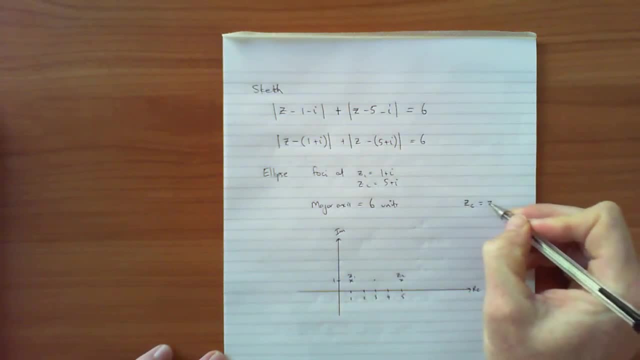 then you could say: ZC, C for centre is Z1 plus Z2 divided by 2. in other words, average the two foci. if you average them, you'd get 1 plus I plus 5 plus I divided by 2, which would be: 1 plus 5 is 6 plus 2I over 2. 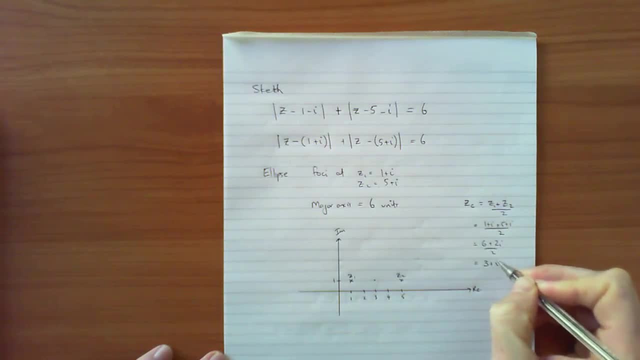 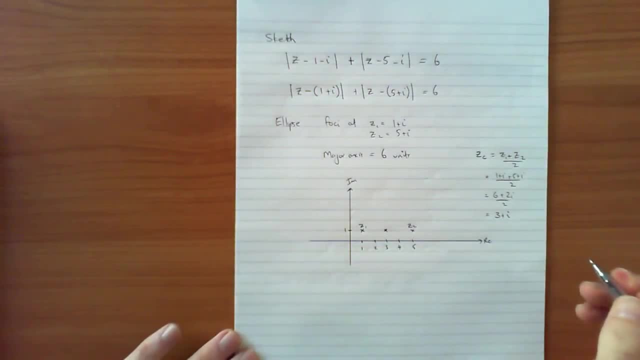 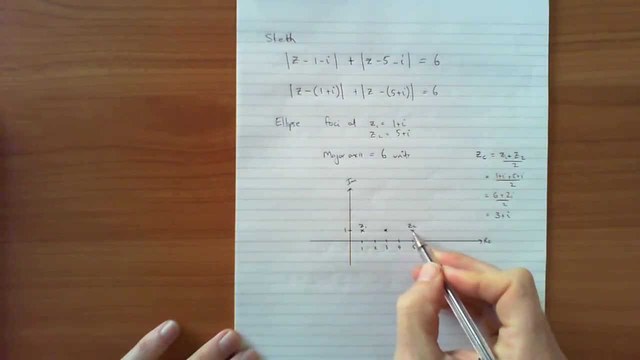 3 units either side. if I go 3 units this way, I'll go 1,, 2, 3, I'll be up to 6, and I go 3 units this way, I'll be back to there. so here are my vertices, indices on my major axis for my ellipse. Now, the only thing here is we don't before we can draw. 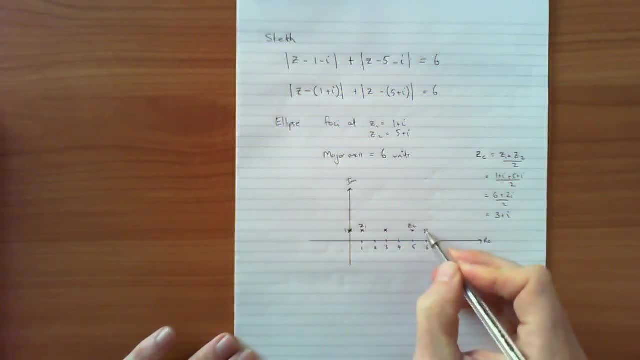 our ellipse. we don't know how fat or how skinny to draw it because we don't have our minor axis, and so we just need to pause for a sec here and and remember or think about how can we work out how far up or how far down, in other words, what's the length of the minor axis in this case? 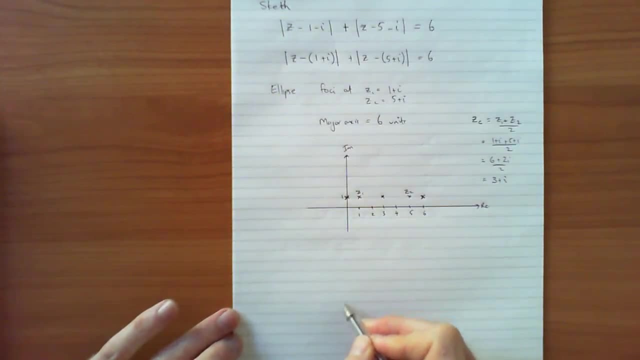 To do that, I'm going to draw another little quick sketch underneath here. okay, so here's just any old ellipse. there's the center, here's the two foci. Now, at the time when, as you're drawing your ellipse, when the string is going up around your pen there and back down, in other words, when 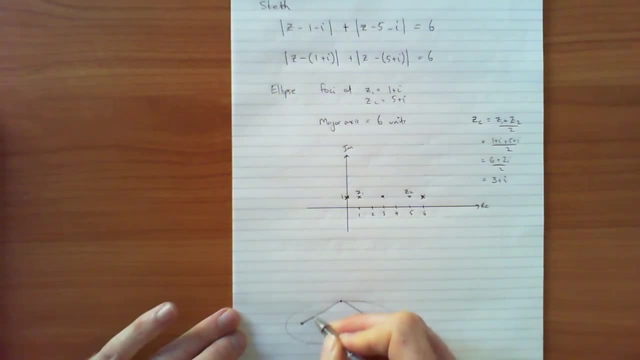 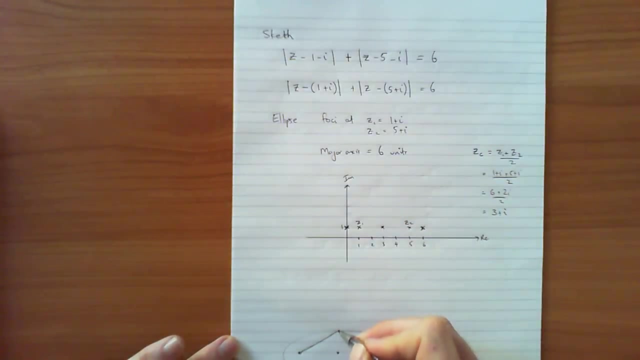 you're directly drawing your ellipse. you're going to draw a little quick sketch underneath here. I'm going to draw a little right angle triangle here. Now, remember, this is the foci. they've got to be exactly above the foci. I know that this plus this must be equal to six. Okay, at the moment that. 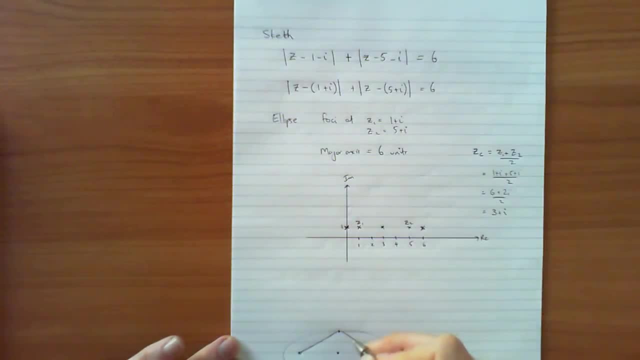 the pen is up here. this distance plus this distance must be equal to six from the equation. Therefore, I know that this distance must be three. Now I'm going to draw a little right angle triangle here. That's the foci, this is the center. What's the distance between the foci and the center? 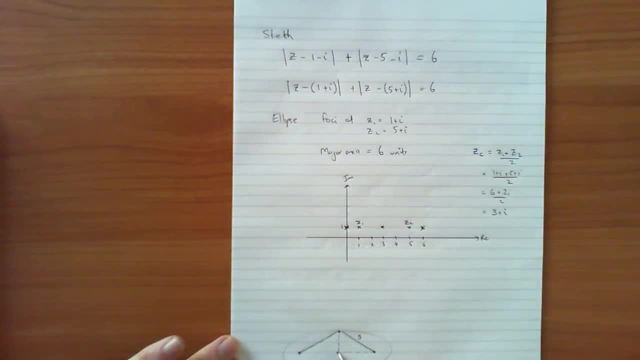 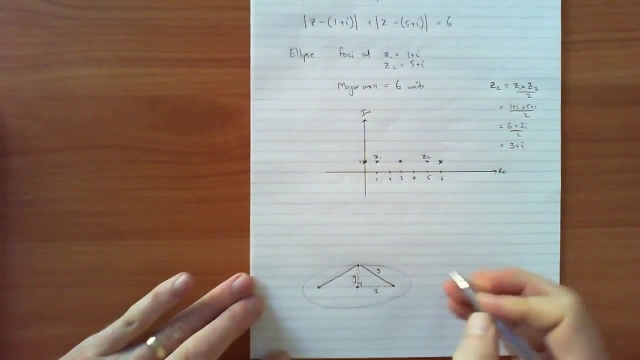 Be careful, it's not three. Okay, that's between the foci and the vertice. Between the foci and the center is two units. Now I can use Pythagoras rule to find that distance there. Okay, I can use Pythagoras rule to find that. So I know that two squared plus y squared equals. 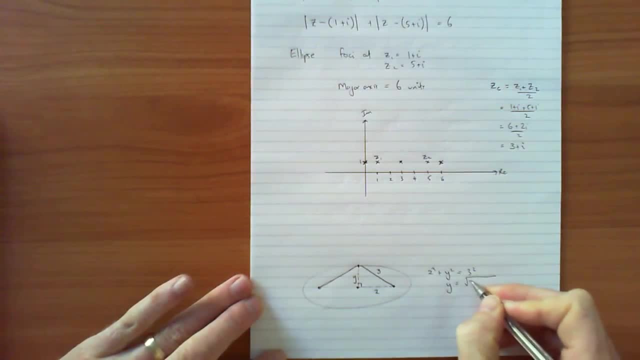 three squared. So y will equal the square root of three squared minus two squared, or y will equal the square root of nine take four, which is five. So I now know that my semi-minor axis is square root five units. Now you know that the square 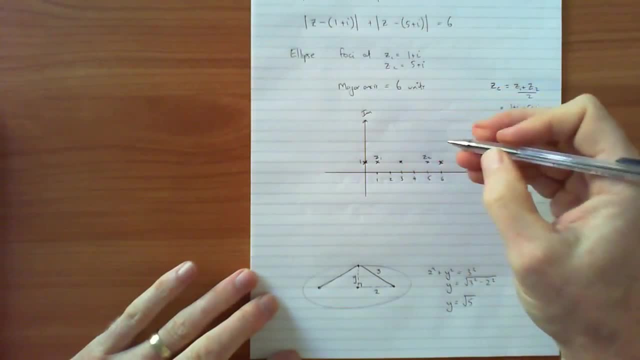 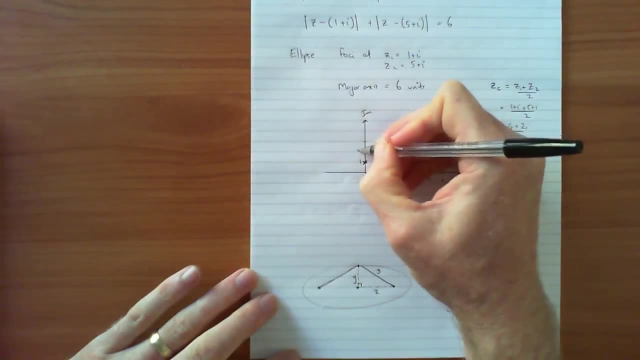 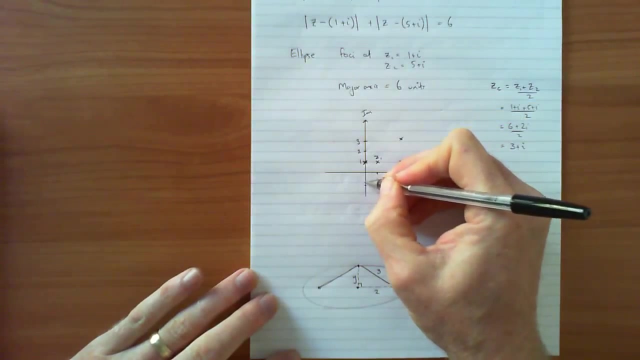 root five is going to be a bit over two. So I'm going to come up square root five units and I'm going to go down square root five units. So I'm going to be down about there And I can label that point. I can label it as three. 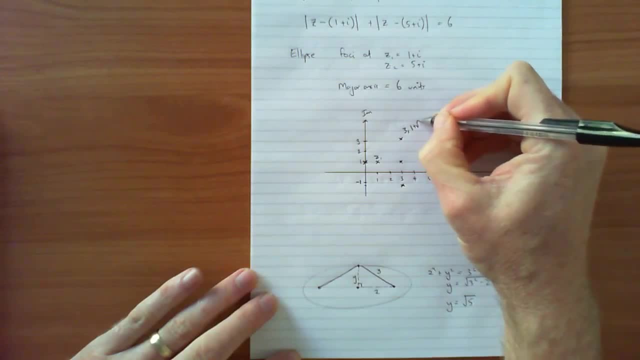 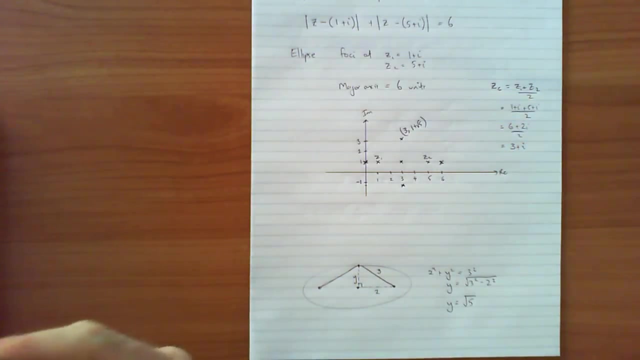 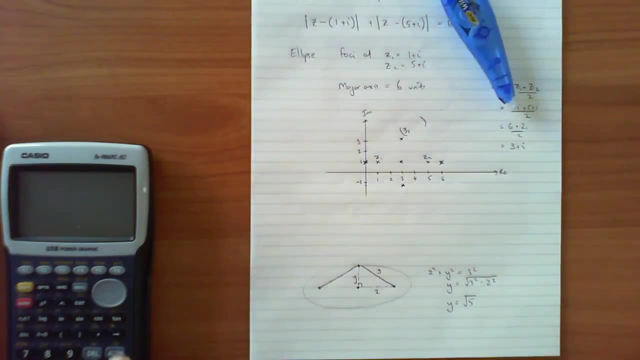 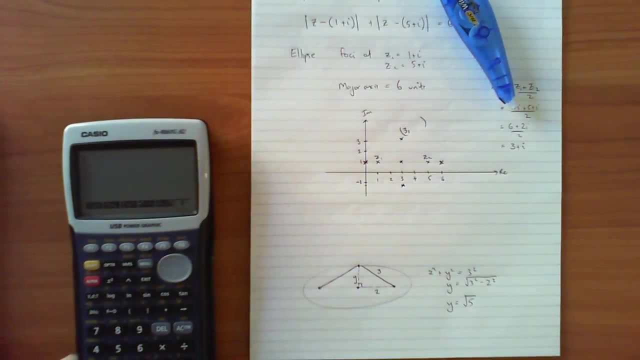 one plus square root five, And down here it will be and you can actually get your calculator and it might be easier to get your calculator and actually write that as a decimal. We'll take that out. So One plus square root five, three point two, three. 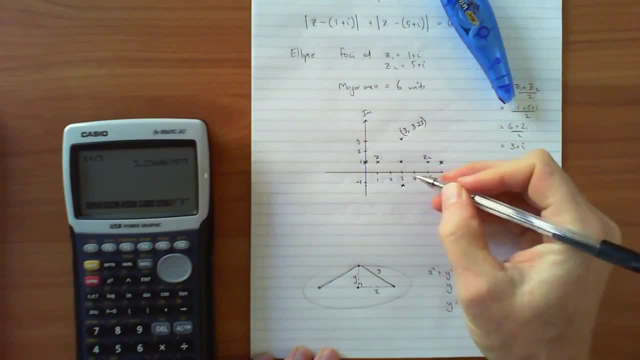 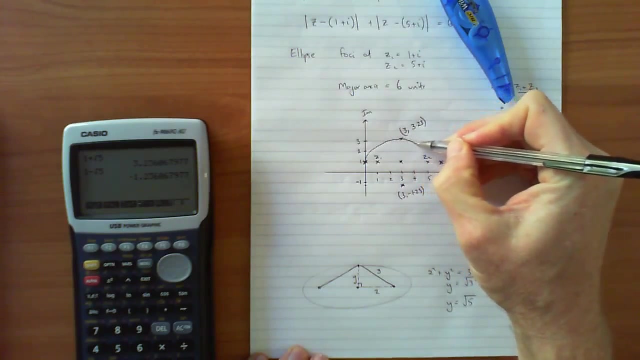 And down below It will be one takeaway: square root, five, Unquote: Subtract them, that will help me a lot. Okay, So I, Yes, Subtract them. Subtract them, it will help me a lot. And now we can draw in our ellipse. 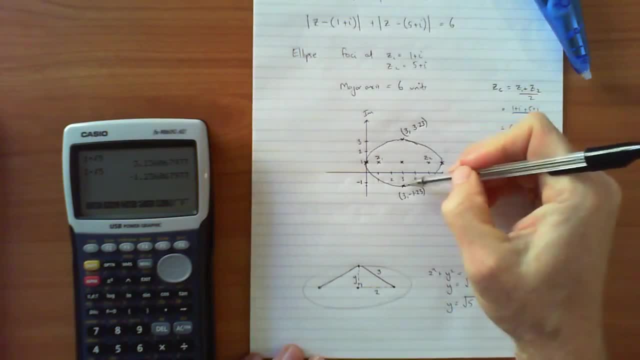 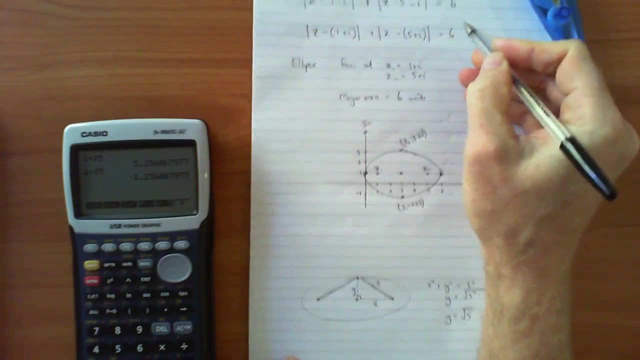 There it is. So the hardest part of drawing the ellipse is actually working out the minor axis, which I strongly recommend you draw a little diagram like this to help you work out your semi-minor axis. Just keep in mind that that distance plus that distance was our value of 6 here. 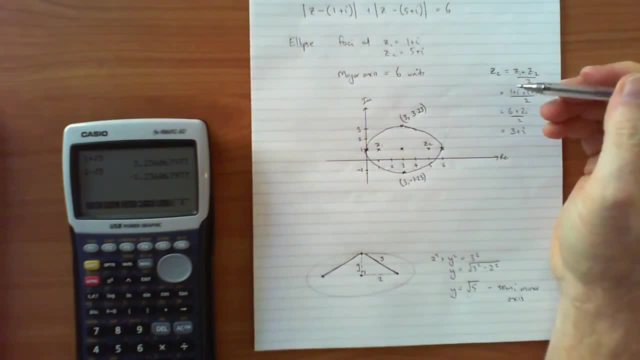 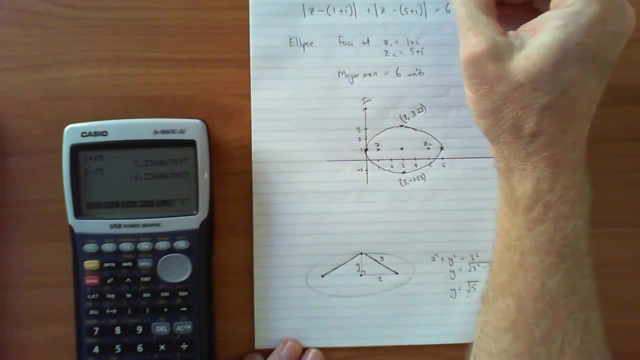 And so that is sketching ellipse. By the way, if we were sketching a region, if we turned this into a region, if that was a less than or equal to sign, then we would shade inside the ellipse. If it was a greater than or equal to sign, we would shade outside the ellipse. 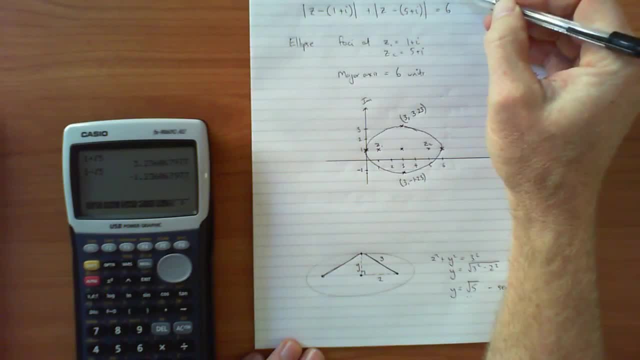 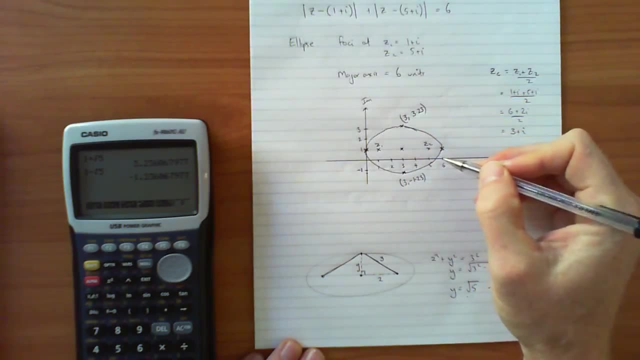 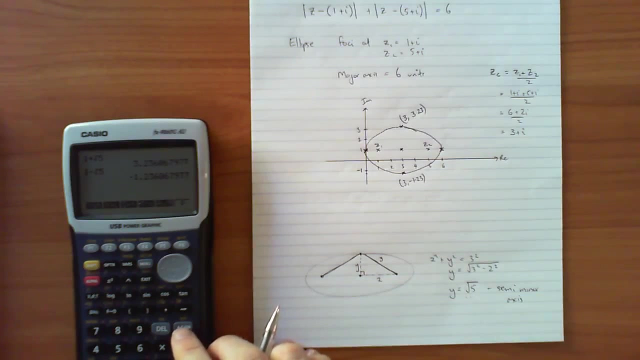 If it wasn't an equals, if it was just a less than, if it was just a less than, then we would dot the boundary and we would shade inside. if it was just a less than. So we can combine what we were learning before with regions, along with ellipses. 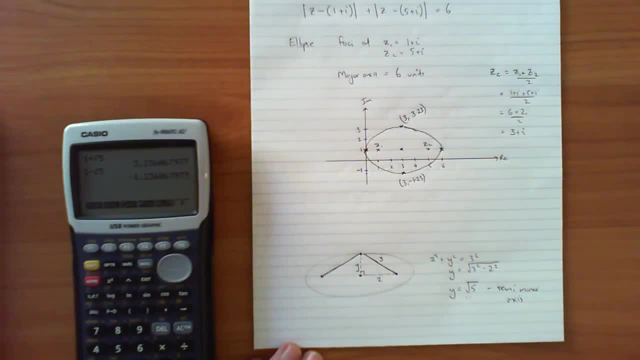